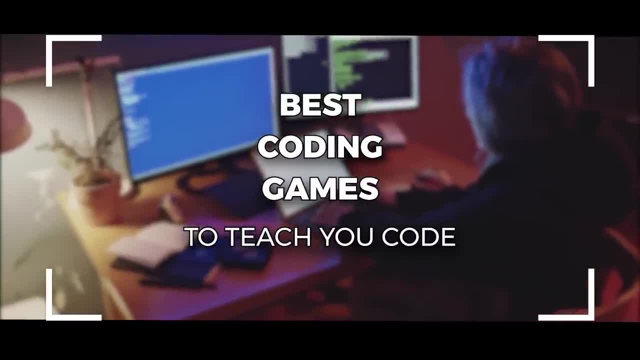 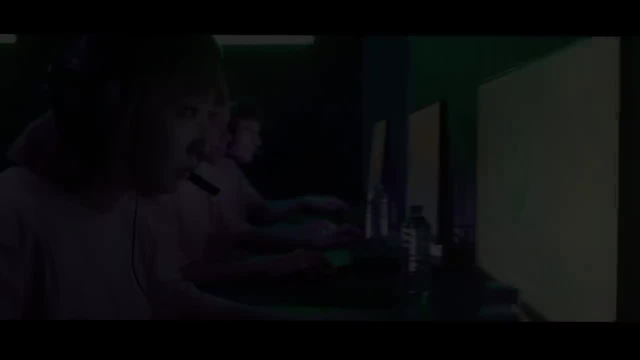 isn't going to teach you everything, but it can be an incredible way to practice the skills. In no particular order, let's start with our first game. First up, Robocode. Robocode is a complex programming game that lets you code robot. 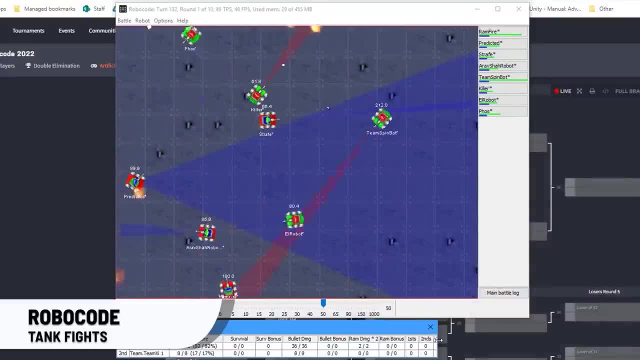 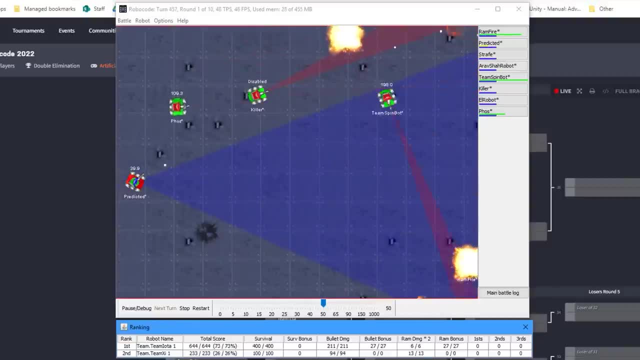 tanks and pit them against each other. Your role is to write the artificial intelligence that drives your robots to success using real languages like Java, Scala, C-Sharp and more. The Robocode installer comes with a development environment built in Robot Editor and Java. 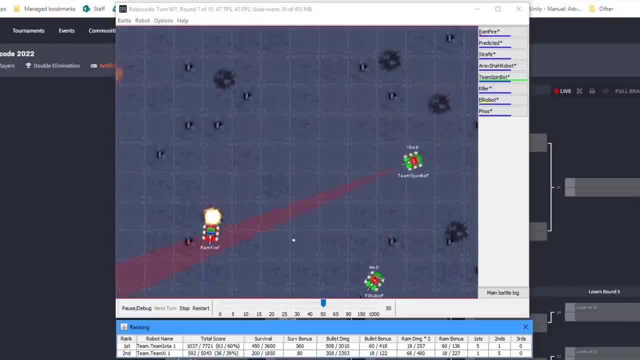 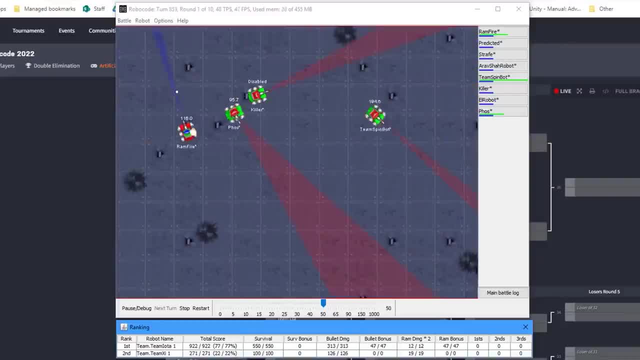 updated and maintained, helped along by the fact that it's open source and addictive. In addition to explicitly teaching programming concepts like sequencing, loops and conditions, lessons incorporate storytelling, arithmetic, science and art. Coming up next? Code & Game. Code & Game is a game-like web app. 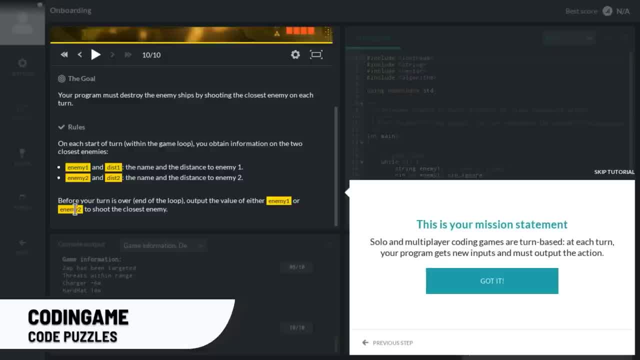 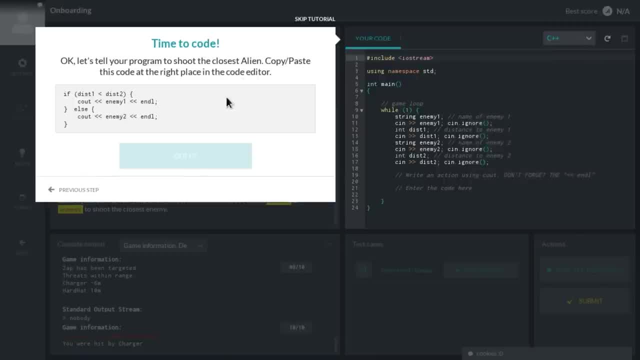 where you solve puzzles and challenges by writing real code. There are more than 25 different programming languages that are supported, including Java, C-Sharp, Python, JavaScript, Lua, Go, Rust and more. Each puzzle or challenge in this web application. 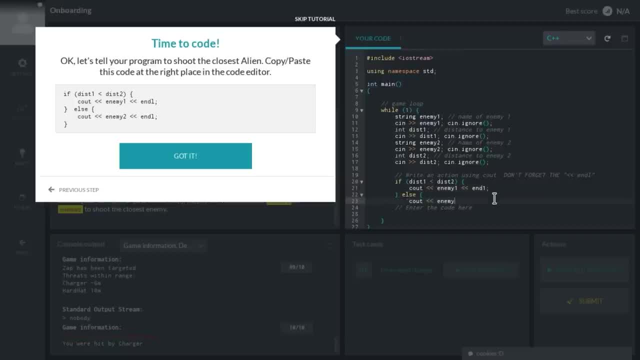 has a unique and exciting theme. For example, you may have to program the turret to shoot down airships that come too close. save your ship or race your car to win some galactic championship. These themes surely kick up the fun factor and make coding more fun. 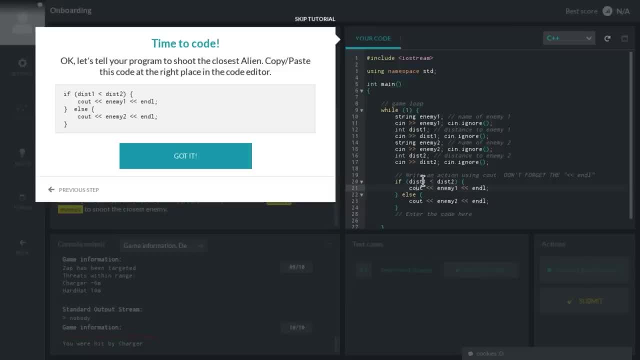 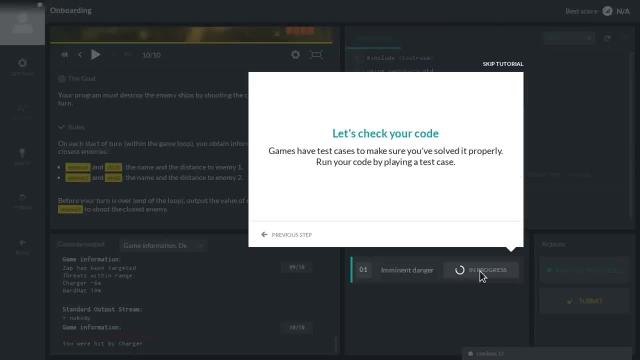 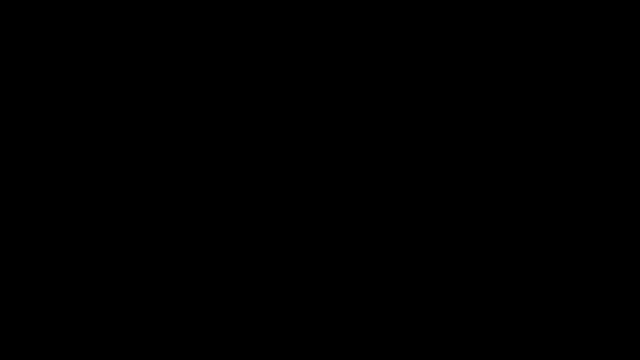 It can improve programming abilities and problem solving skills. Many treat it like a game only, but you will really see improvement in your coding skills. It's treated like a subject of school and students have to derive the logic and generate the output Coming in. next, Code Monkey. Code Monkey is a fun and educational game-based environment. 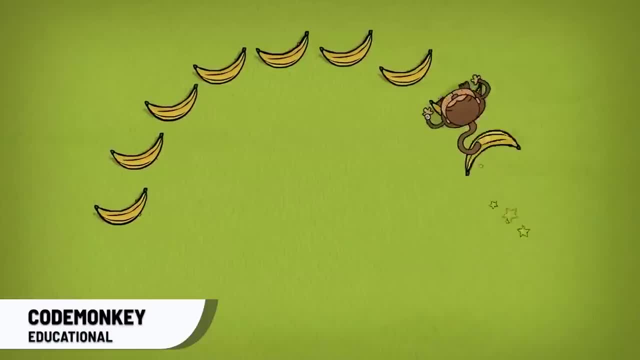 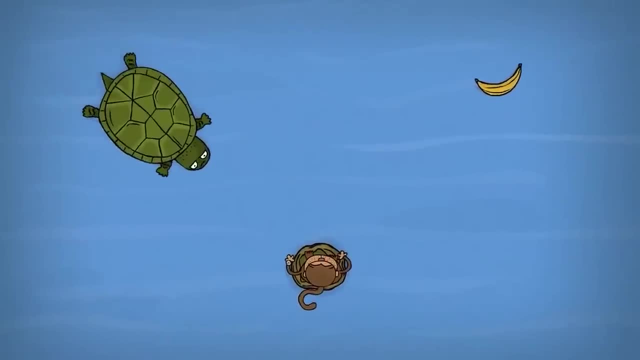 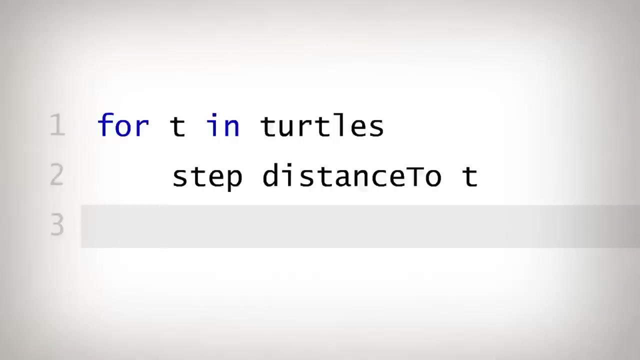 where even kids can learn to code without any prior experience. After completing Code Monkey, you can learn to code in a game-based environment where even kids can learn to code without any prior experience. This environment also offers educational resources for students of different grades and experience levels, From Code Monkey Junior to Banana Tales. 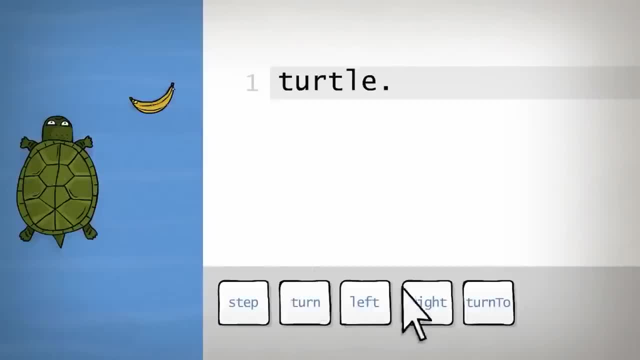 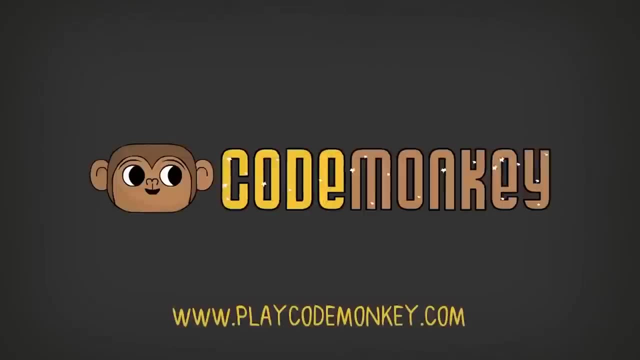 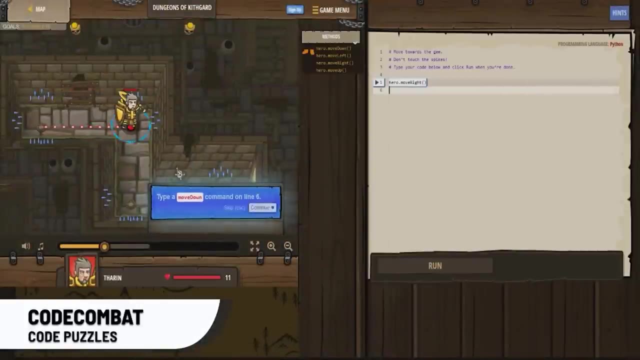 students not only learn coding basics, but also how to code in real programming languages. Through Code Monkey, you can develop the necessary skills for the future while having fun. Up next, Code Combat. Code Combat is another web app for game-like puzzles and challenges. 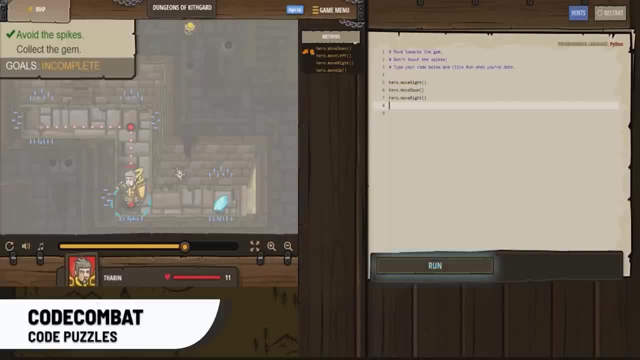 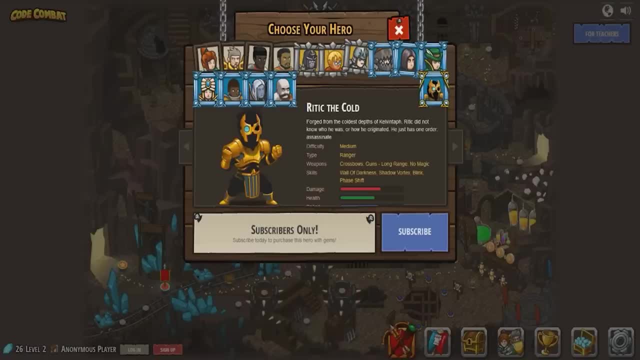 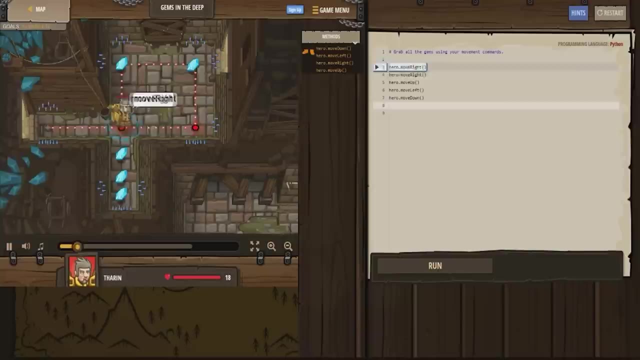 that can only be solved by writing code. Code Combat has a significant educational angle, with a classroom addition that teachers can use to help their students learn how to code. The web app offers three different course paths for you to pursue, including computer science, web development and game development. Here you can learn Python, JavaScript, CoffeeScript. 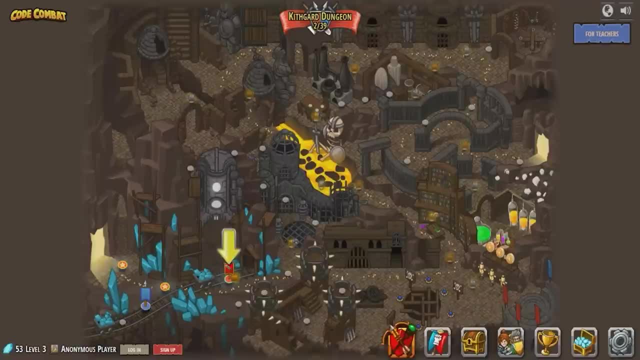 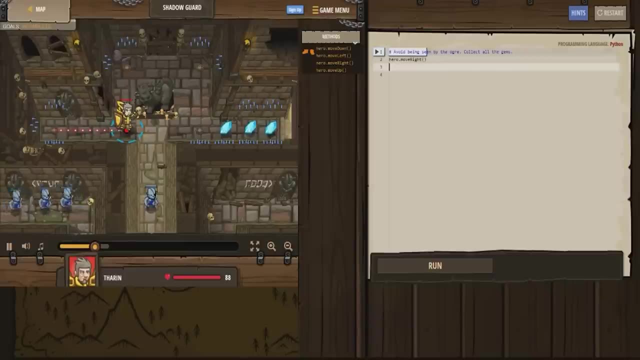 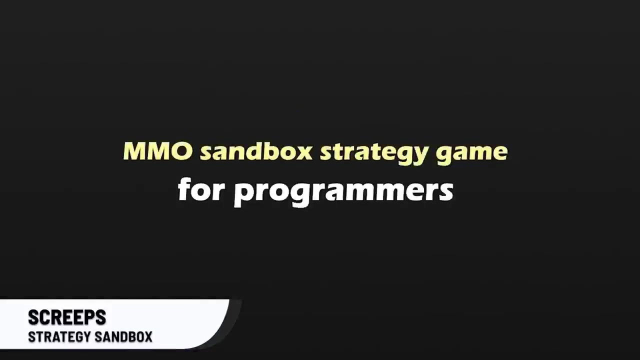 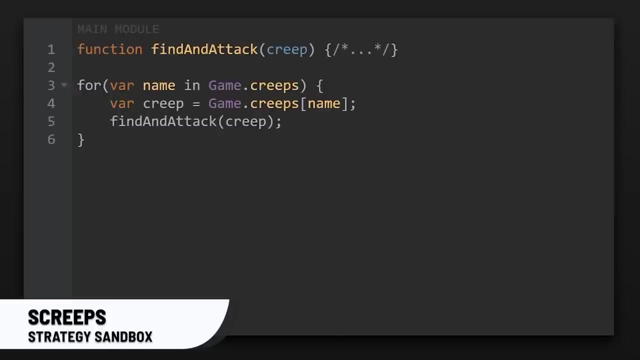 or the Lua game. This web app is mainly aimed at teachers and students, but anyone can play. If you're unfamiliar with Python, JavaScript or HTML, just play the game in advance. You'll learn too. Up next Screeps. Screeps is an MMO sandbox strategy game for programmers. This is a serious 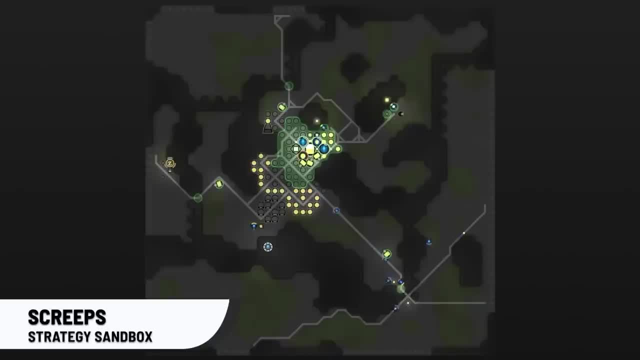 programming game that assumes you already know some basic programming. You can control your units using real-life code and you can also control your units using real-life code. This is a serious programming game that assumes you already know some basic programming. You can control your units. 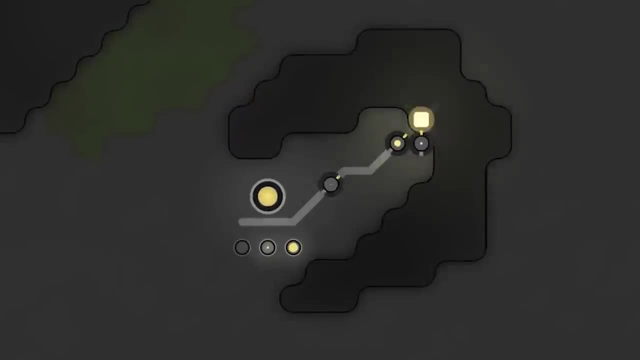 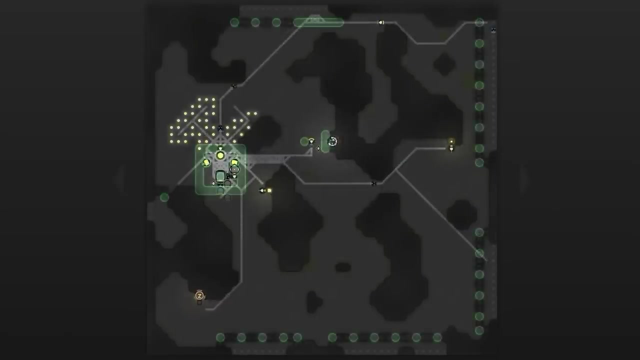 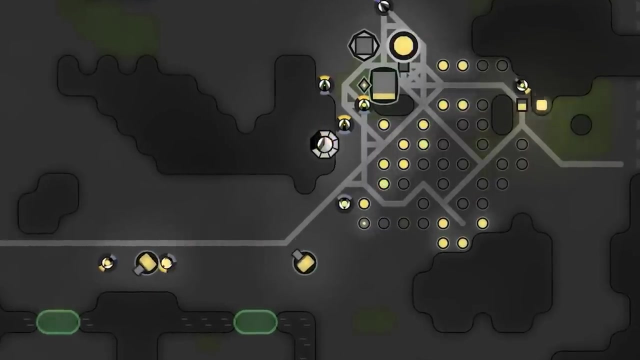 programming languages like JavaScript. You can even compile languages like C++ and run them through WebAssembly. Using actual programming instead of pseudolanguage actually allows the players to focus on better coding habits and makes practice fun. Screeps came out back in 2017. 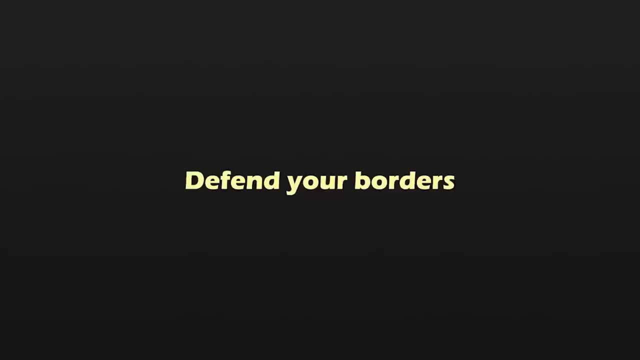 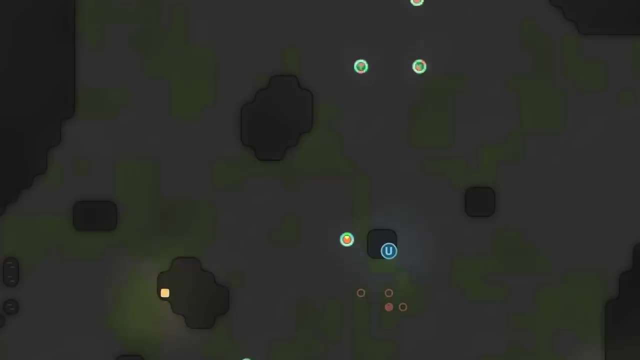 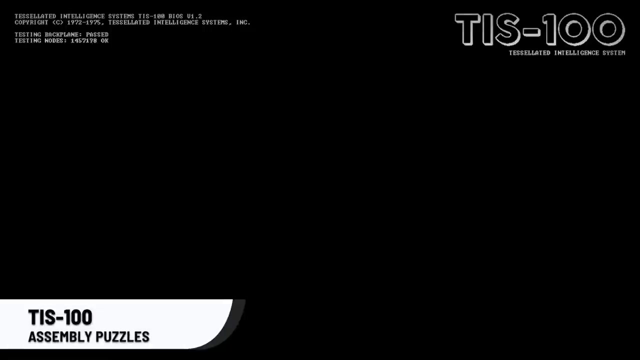 and is still actively maintained. It's currently sitting at an 89% positive rating on Steam, with more than 1,000 reviews, which makes it one of the more acclaimed games on the web. Screeps is a game that's been on the entire Steam platform, Up next TIS 100.. It's a programming puzzle video. 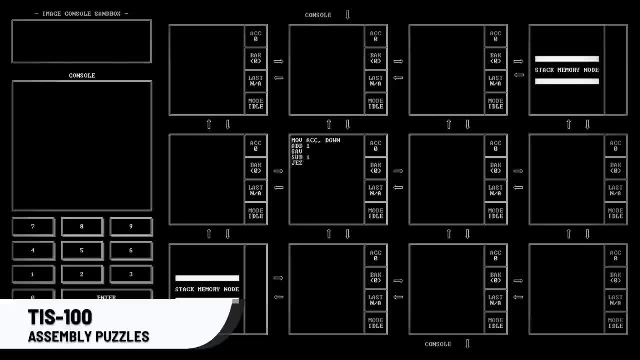 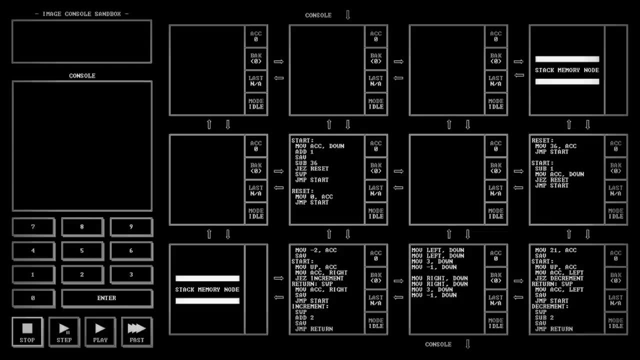 game developed by Zachtronics Industries. It's the assembly language programming game you never asked for. It says so right there on its title. TIS 100 is a video game like no other, forcing you to learn and use mock version of low-level assembly code to solve its puzzles. The game has 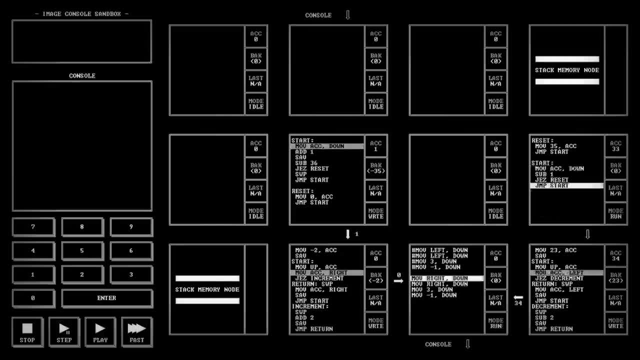 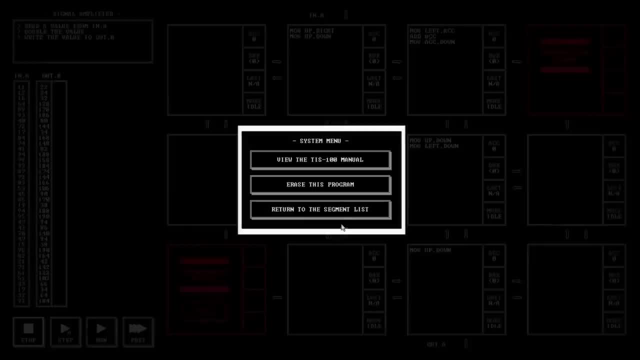 the player develop assembly language code for the game and the game has the player develop assembly language code to perform certain tasks on a fictional, virtualized 1970s computer that has been corrupted. This game is not a joke. It's difficult, open-ended and it has incredible 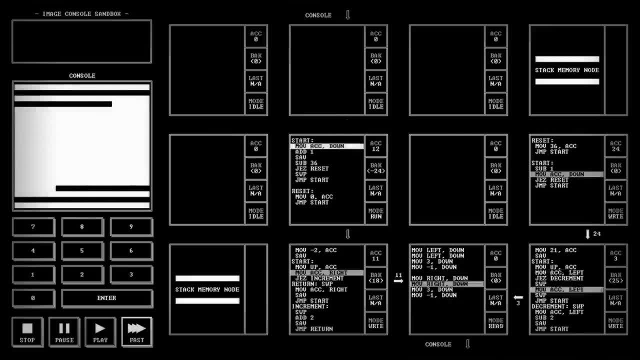 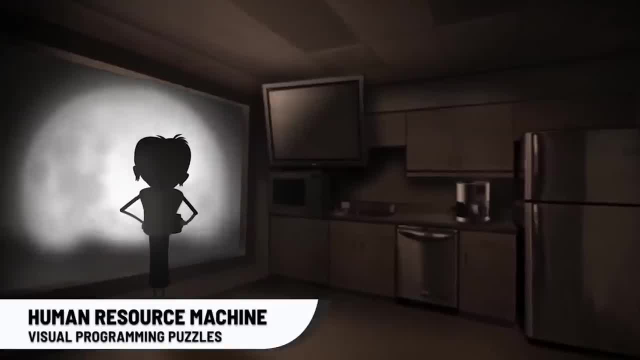 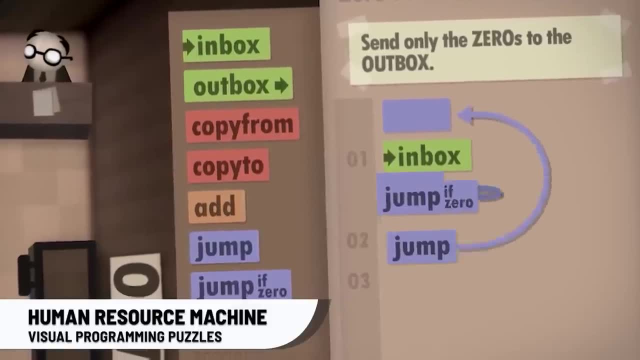 replay value as long as you don't become so frustrated and confused that you uninstall, in a fit of rage, Coming in next, Human Resource Machine, a visual programming-based puzzle video game developed by Tomorrow Corporation. Human Resource Machine uses the concept of a corporate office worker assigned to perform tasks. 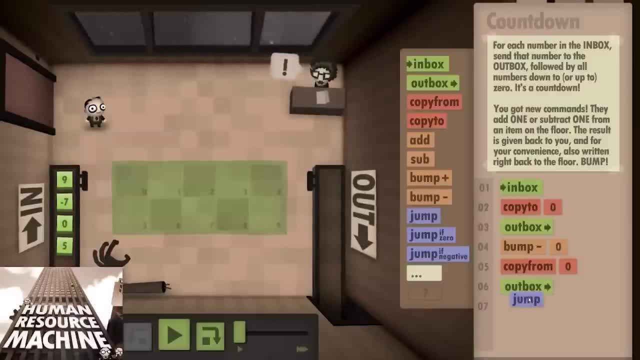 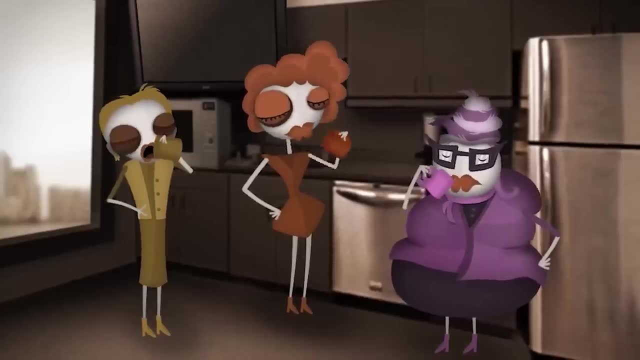 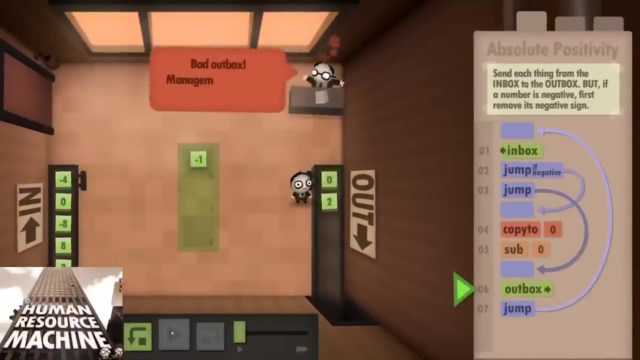 that involve moving objects between an inbox and outbox and to and from storage areas as a metaphor for assembly language concepts. The player works through some 40 puzzles in constructing a program to complete a specific task. In a sense, this game is all about puzzle solving through visual. 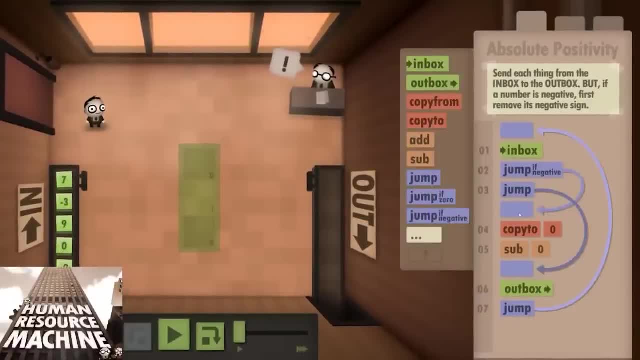 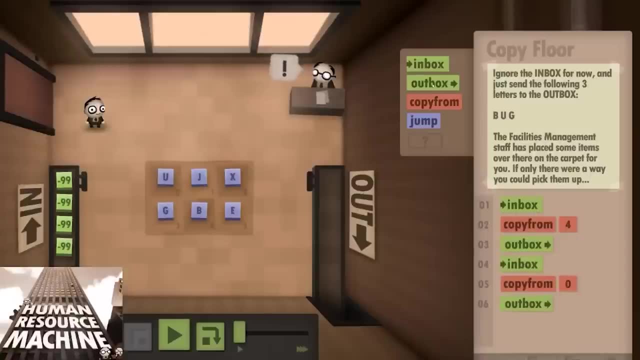 programming, even going as far as to touch on concepts like logical flow and memory management. But presented in an easy-to-digest, office-themed way, it's a great game for exercising your programmer's brain and may even make a good coding game for kids too. 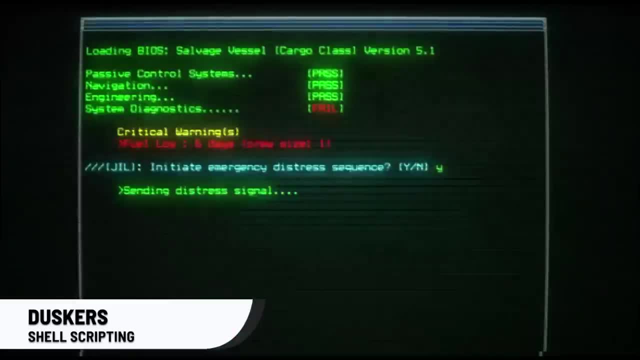 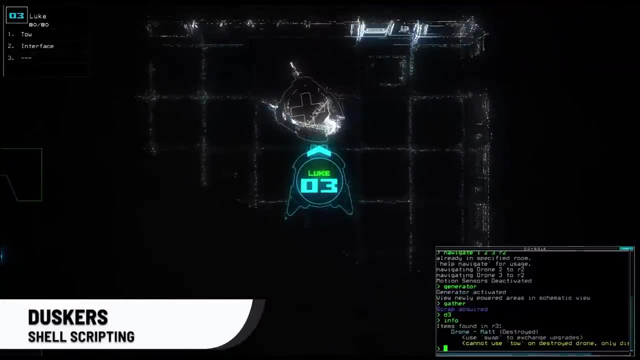 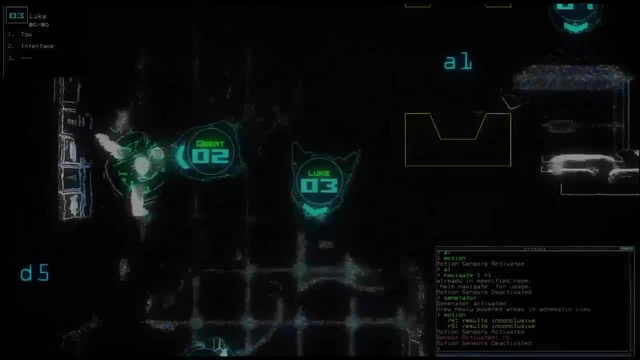 Coming in next Duskers. Duskers is a game that resembles shell scripting. You play as a programmer who is stranded in space and running low on supplies. You have to dock with abandoned space vessels and then scavenge them, But you can't interact with these ships directly. 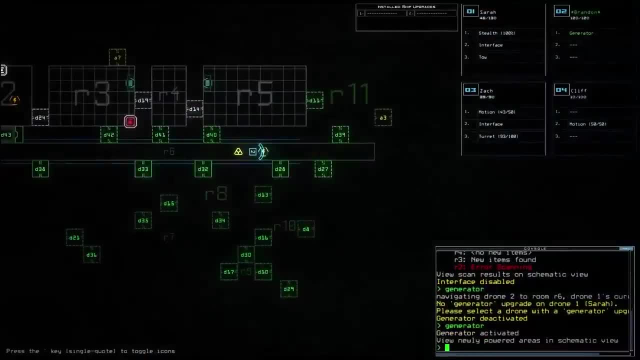 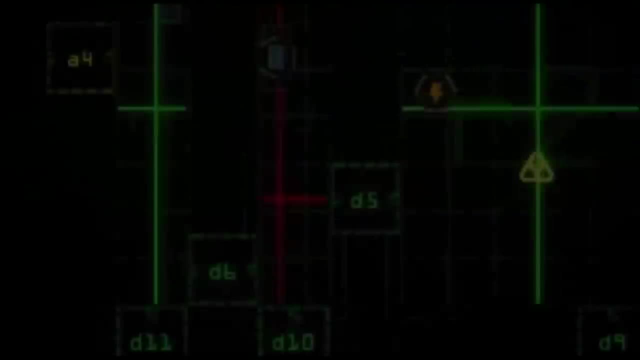 Instead, you control a team of drones, each with their own abilities, and tell them how to explore these ships. There are also monsters on the ships that will destroy your drones if you're not careful. This game is controlled entirely by typing into a command line interface, Because 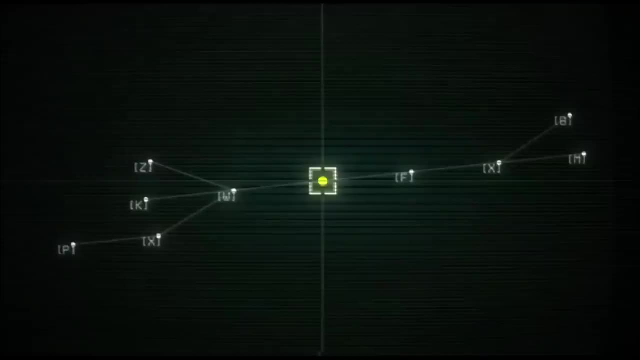 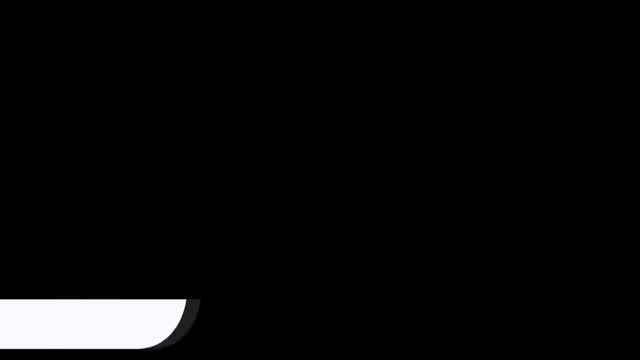 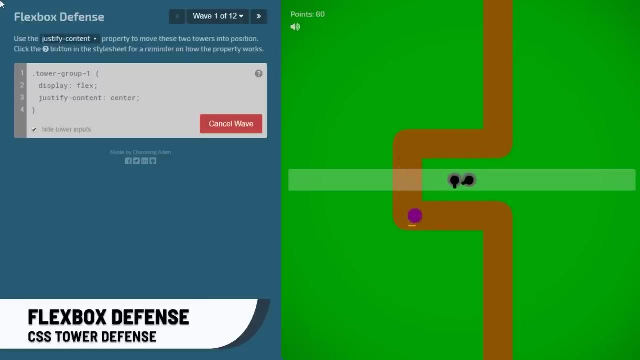 the game is real-time in nature. this can lead to some intense moments of rapidly typing commands as you try to save your drones from danger. Up next, Flexbox Defense. This is a tower defense game that involves you protecting yourself using Flexbox-based commands.